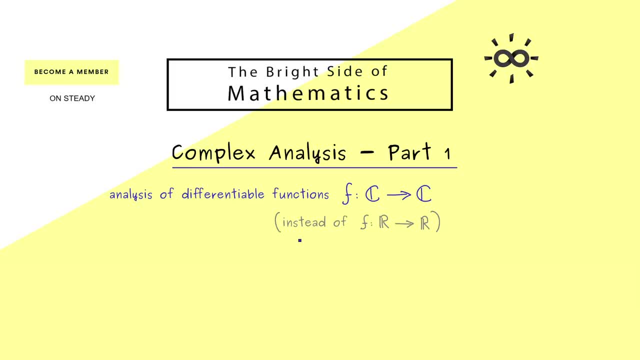 in the definition of differentiability, And from that a lot of strong theorems will follow, which indeed don't hold true. However, since the real number line r is a subset of the complex plane c, we can often apply these theorems, even if we just consider some real functions, For example, a real problem where 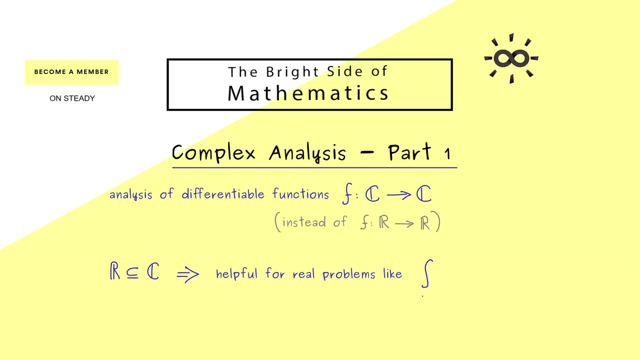 complex analysis can be really helpful is calculating an improper Riemann integral. This could be the integral, from minus infinity to infinity, of the function x times sine of x divided by one plus x squared. Now, indeed, finding an antiderivative of this function is really, really hard. However, just calculating the whole integral with complex analysis. 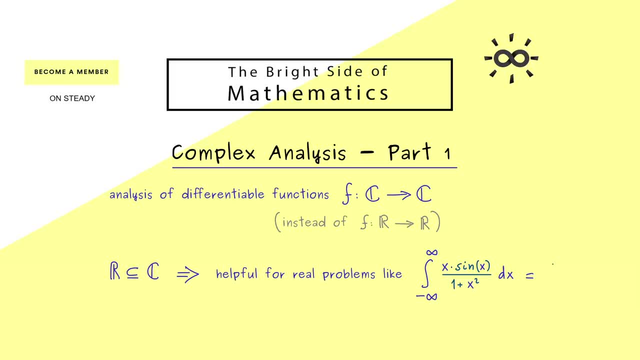 is surprisingly simple. Indeed, the result we find is a number slightly larger than one, namely it's pi divided by e. How to do this simple calculation here, we will learn in this course. However, of course, first we have to start with the basics, And i already told you. in contrast to 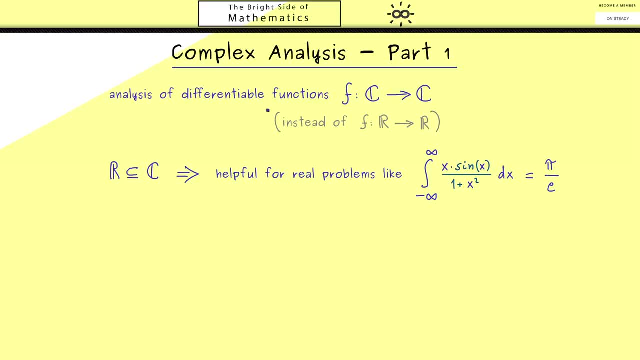 real analysis, we immediately start with differentiability. The definition first looks the same as in real analysis, but it is way more powerful, as we will see Now. in order to understand this new definition, you will need to know some basic facts. First, you need to know how to work. 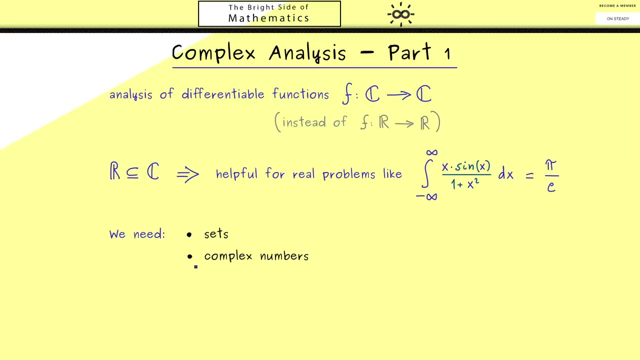 with sets, And of course you also need to know how to work with sets. And of course you also need to know how to calculate with complex numbers. If you have problems there, you find everything you need in my start learning mathematics series. This is a whole playlist. 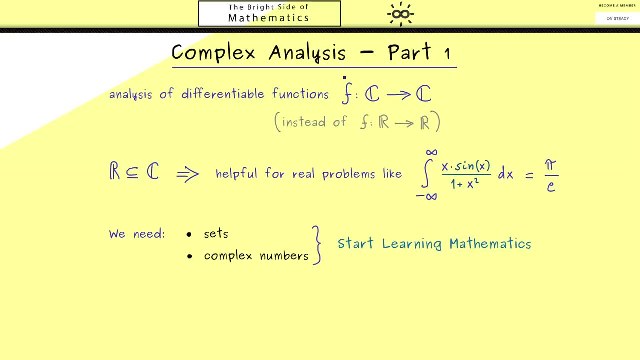 that covers all the basics you need for this course here. In addition, it's also good if you already have a basic knowledge of some topics of real analysis. For example, you should know what a continuous or a differentiable function from R to R is. If you already have a basic, 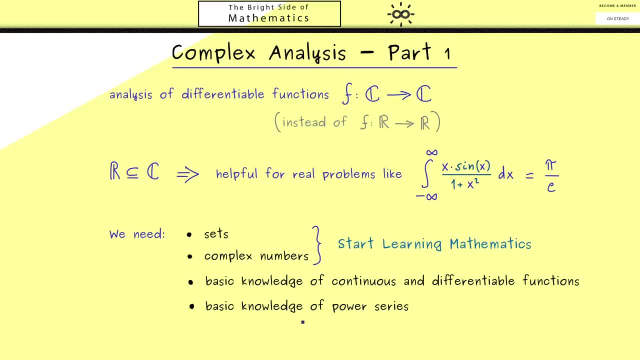 knowledge of some topics of real analysis. for example, you should know what a continuous or a differentiable function from R to R is. Also, it could be very helpful for you if you already know what a power series is For all these topics. of course, my real analysis series can help you. 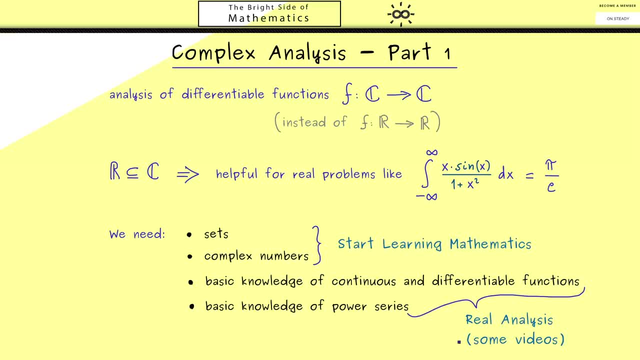 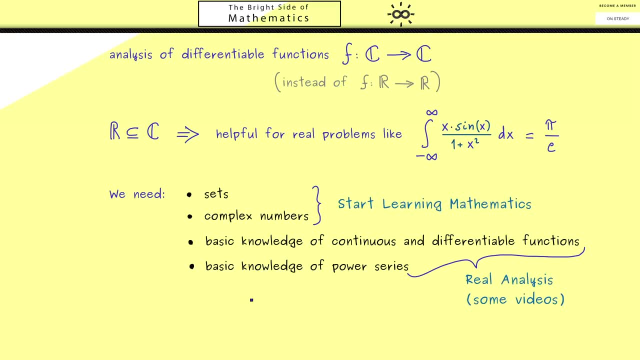 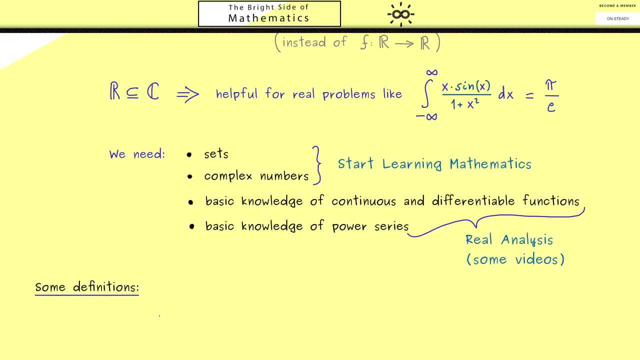 However, you don't need to watch the whole course. Some videos about these topics might be sufficient. Okay, by knowing this, i now think we can start with the course. The first part will be about some definitions we will definitely need throughout this course. First, i can tell you the complex numbers form a set with a distance function. Formally, we call: 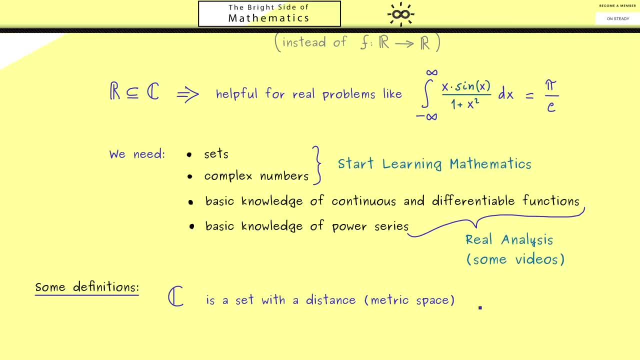 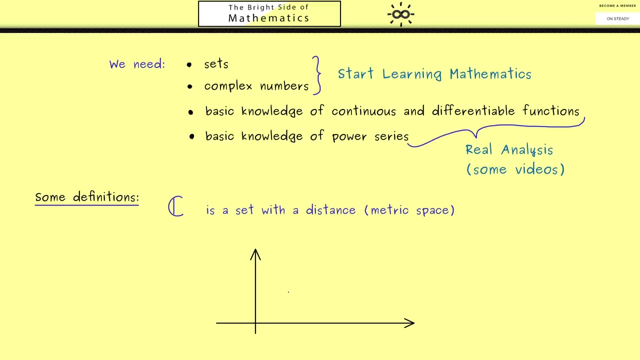 such a construction, a metric space. but don't worry, it's not complicated at all. It just means that the distance between two elements of the set makes sense And of course we can immediately visualize this in the complex plane. This means that a complex number, z, can be found in this plane. 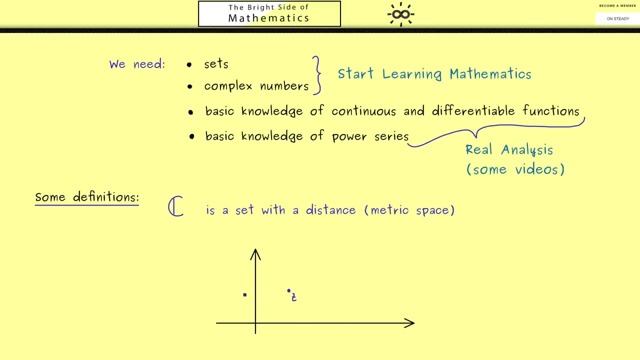 On the x-axis, we find the real part of z, and on the y-axis, the imaginary part. Now you can imagine that we have a second complex number here, we call w, And now what we want to do is to measure the distance between both points. Indeed, this is what we calculate with the absolute. 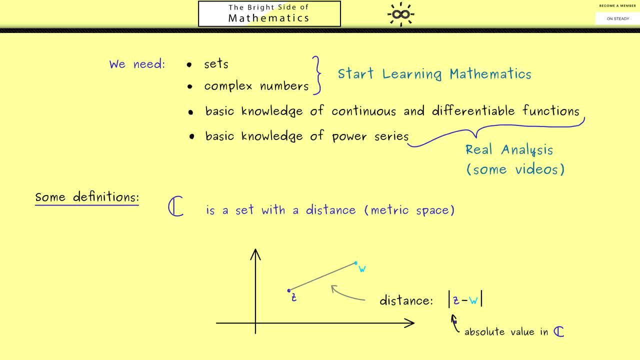 value in c, And what we need is the absolute value of the complex number z minus w. Now, such a notion of a distance is important, because with a distance we can say what a convergent sequence is, what limits are, and so on. Otherwise we wouldn't be able to say that a 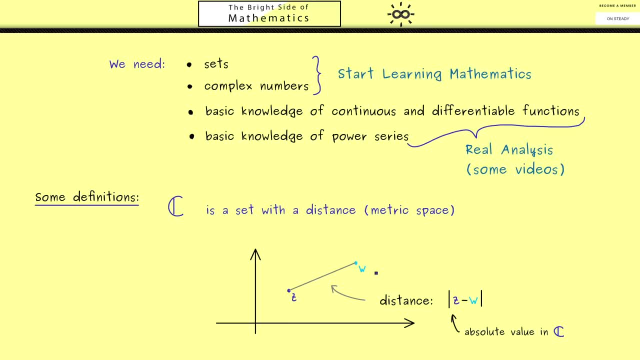 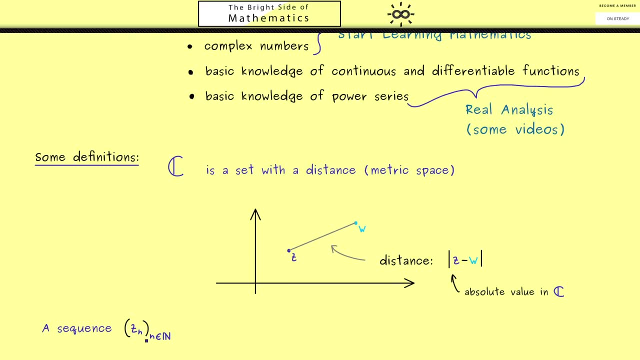 sequence gets closer and closer to a given point. Indeed, we have to measure this closeness. Hence, now we are able to talk about sequences of complex numbers and convergent sequences. So a sequence of complex numbers is denoted by Zn, where n goes through all natural numbers. 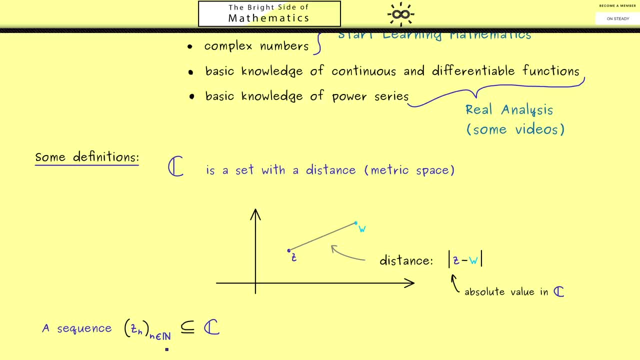 So formally we just have a map that goes from the natural numbers into the complex number c. However, we will always write the sequence in this form, And now we are able to define what it means that this sequence is convergent to a fixed complex number a. 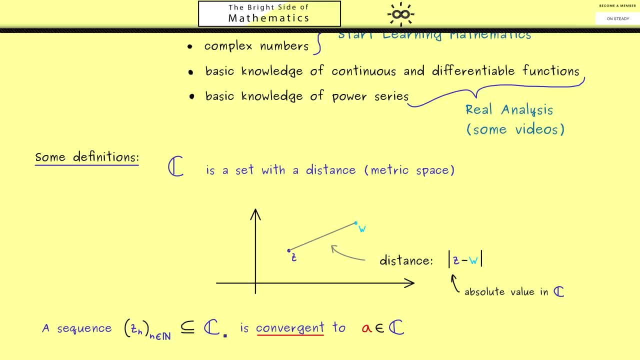 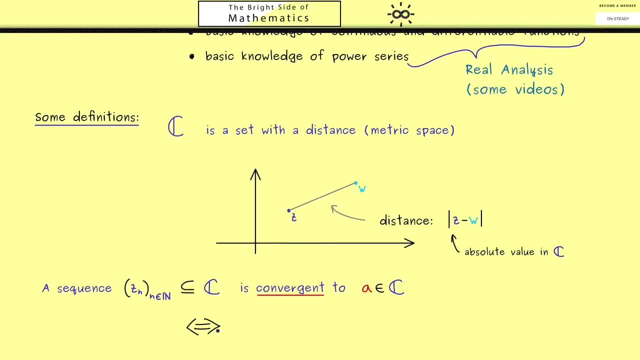 It just means that the distance we can measure between Zn and a gets smaller and smaller until it reaches zero in the limit. This means that we can just look at a sequence of real numbers, Namely the sequence of the absolute value of Zn-a. 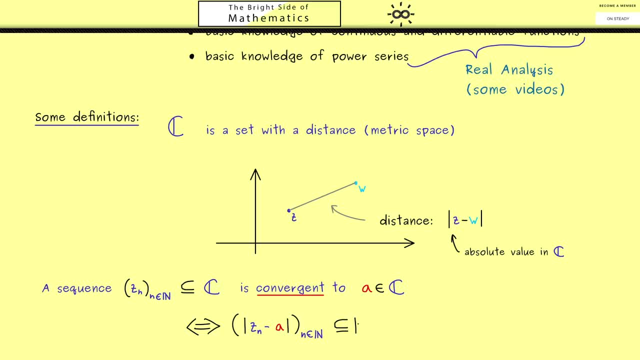 This is, by the definition of the absolute value, a sequence of real numbers, of non-negative real numbers. And now, in the case that this sequence of real numbers is convergent to a fixed complex numbers goes to the limit zero. We call the sequence of complex numbers Zn convergent to a. 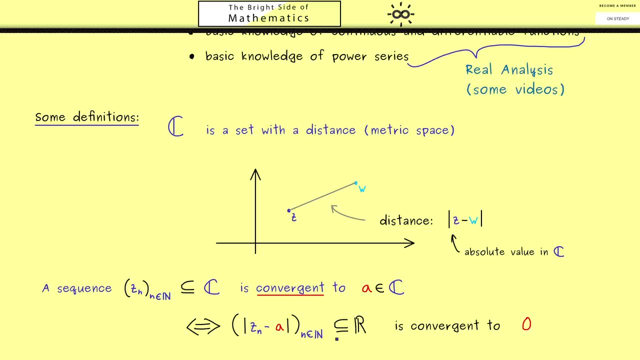 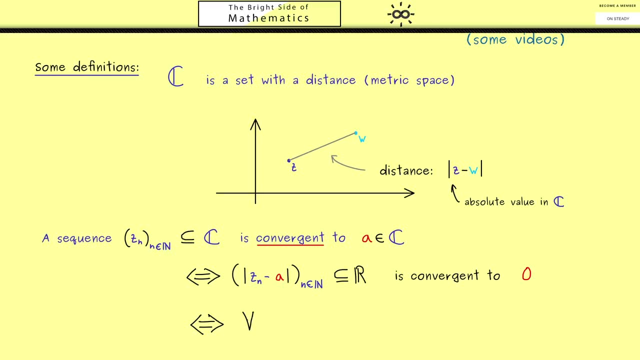 Now, if you don't remember the definition of convergence for real numbers, Lets recall it. So we find that for all positive numbers, we can call epsilon, There exists an index, we can call capital N, Such that for all indices afterwards so n is greater or equal than 0. 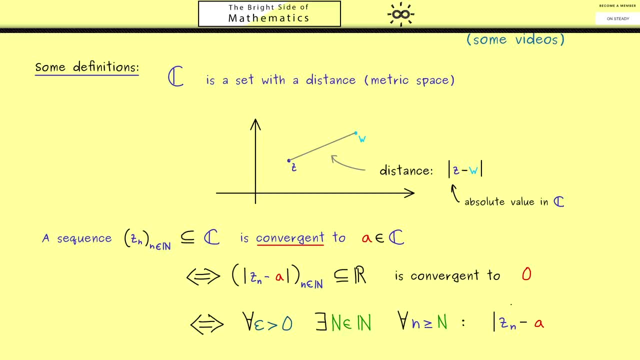 So we find that for all positive numbers- we can call epsilon- There exists an index we can call capital N, Such that for all indices afterwards so n is greater or equal than 0.. then capital N: we get that the distance between Zn and the point A is less than. 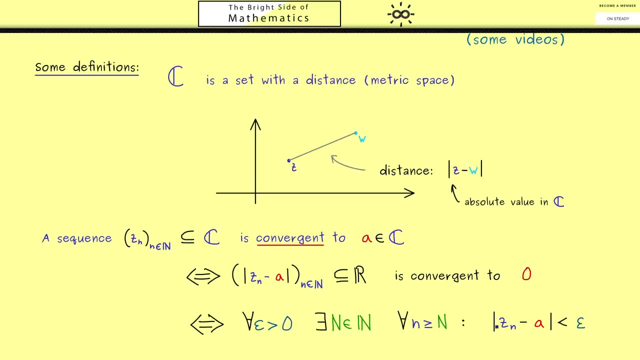 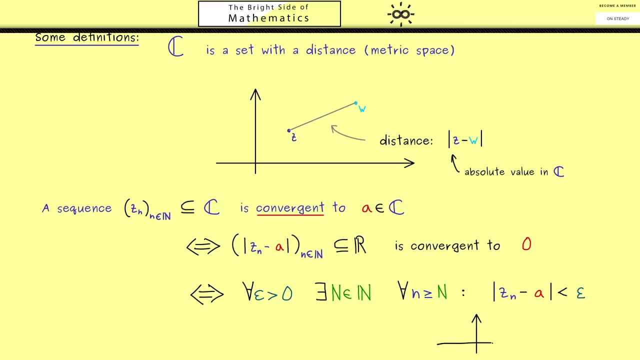 epsilon. So you see, this is exactly the definition we learned in the real analysis. However, now we can visualize it in the complex plane. Now, this formula with the distance less than epsilon means that we can draw a circle around A with radius epsilon. With this we get that eventually. the sequence member Zn. 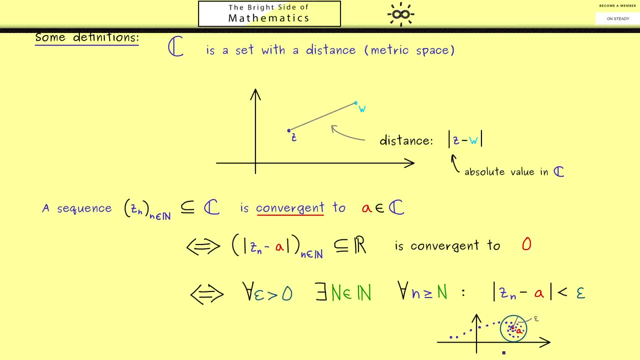 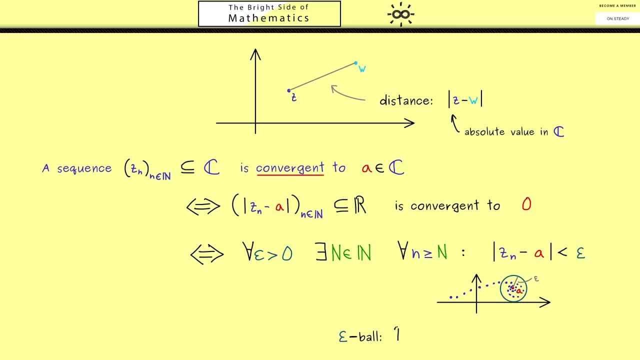 lie inside the circle, So only finitely many can lie outside. And because this whole picture here is so important, we call the inside of the circle an epsilon ball And for the notation we use a capital B with index epsilon. Moreover, the middle point A here we put: 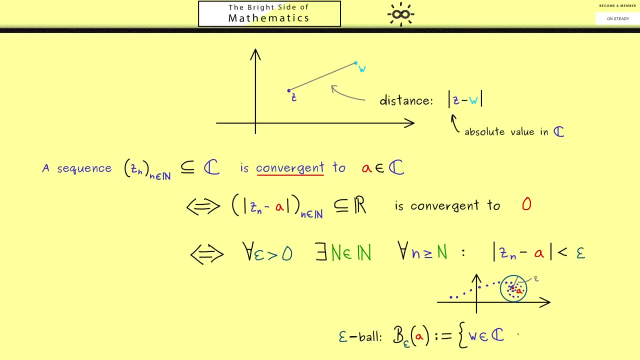 into perspective Now, by definition, this is the set of all the complex numbers, W, with the property absolute value of W minus A is less than epsilon. So this is the definition of an epsilon ball in the complex plane. Okay, because you now know what a convergent sequence in the complex 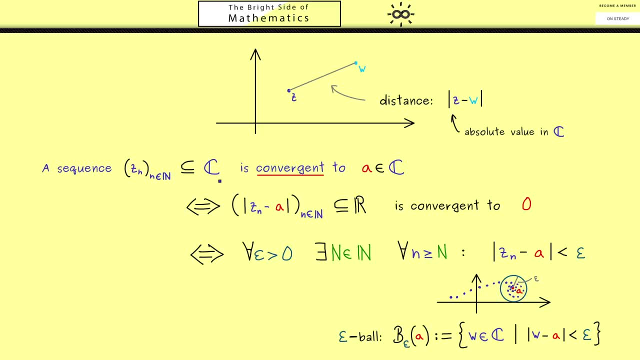 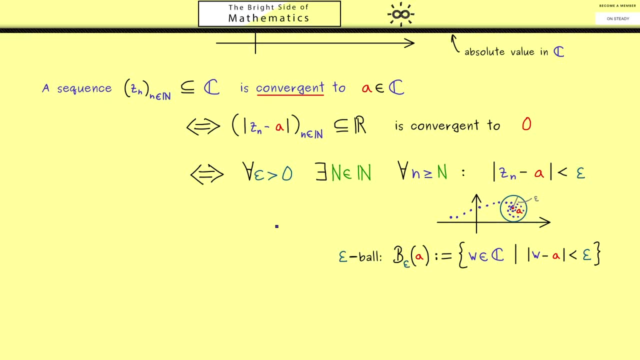 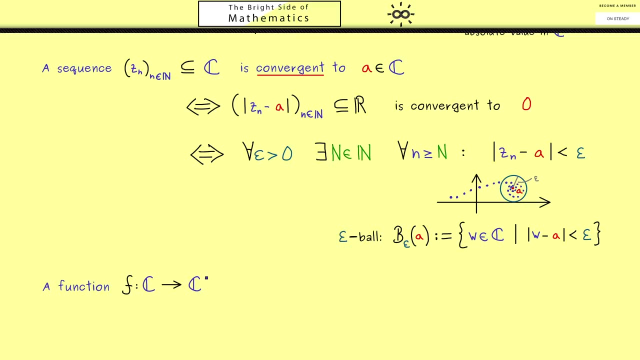 numbers is. you also know what a continuous function between C and Z is. In fact, it has exactly the same meaning as for real functions. Hence, small deviations, small arrows in the input should be translated into small arrows in the output. Indeed, this can be formulated with sequences. Therefore, we say: a function is: